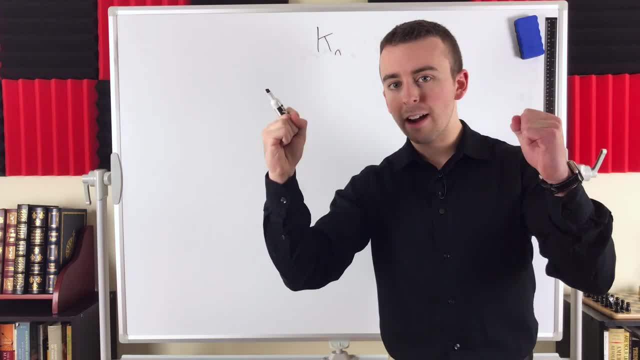 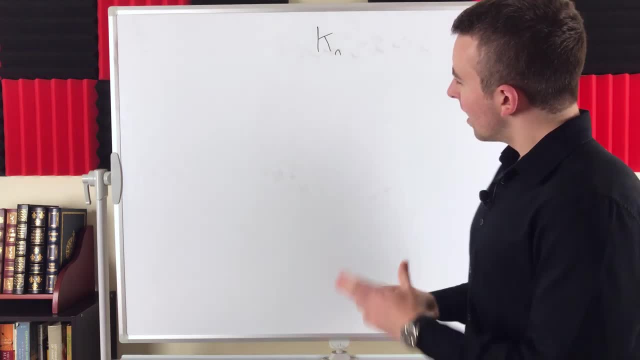 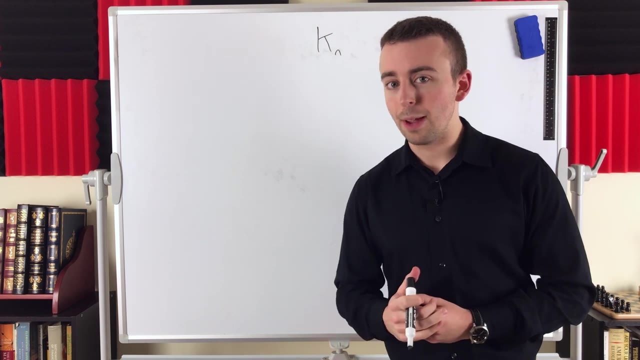 and it's the graph on n vertices, such that each pair of distinct vertices is joined by an edge, So it's got every possible edge. And you would think for a graph like that, where every pair of vertices has an edge, we might be able to find a formula for the number of edges based on the. 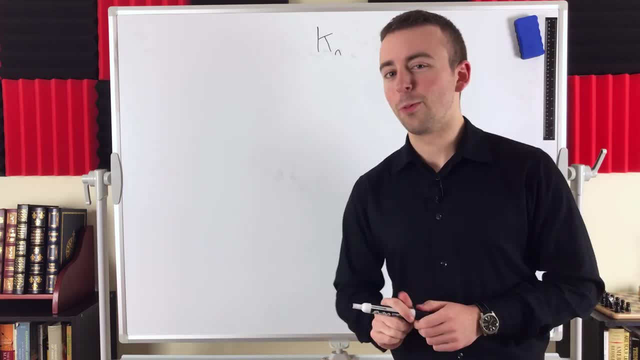 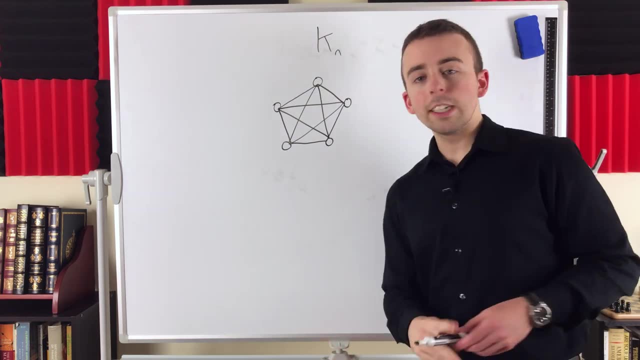 number of vertices. And of course we can- otherwise this video wouldn't exist. So let me draw you a quick example of a complete graph on five vertices. So there's a complete graph on five vertices. You can see every pair of distinct vertices is joined by an edge, and that's what 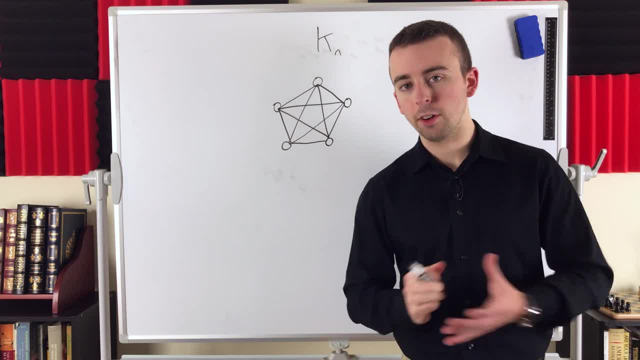 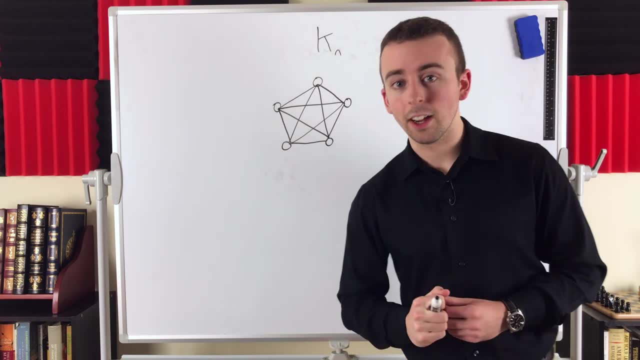 makes it a complete graph. So we're trying to figure out how many edges are in a complete graph. Of course, we don't necessarily know anything about that, but we do know something about the degrees of the vertices of a complete graph. Can you think about what that is? Here's: 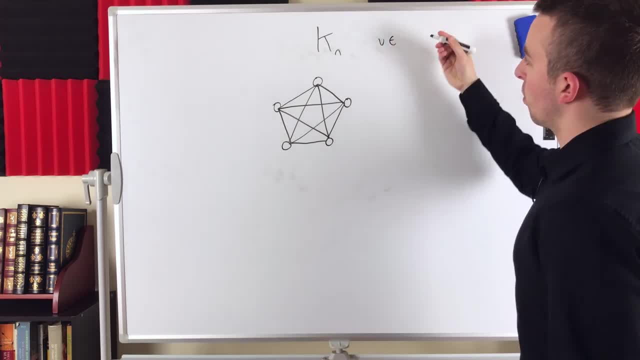 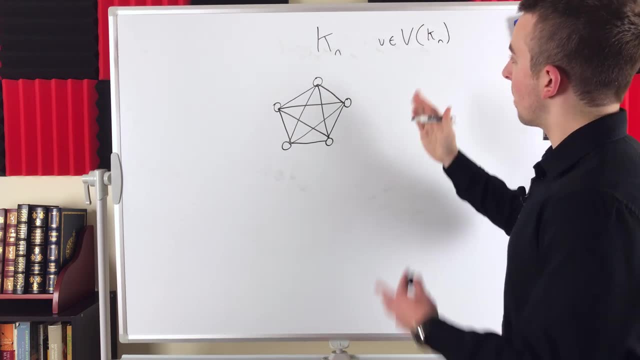 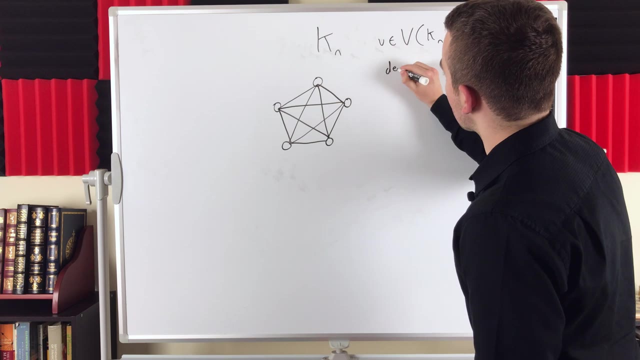 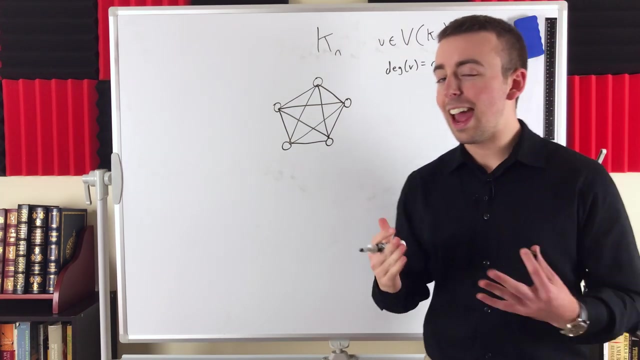 an example of a complete graph. So we'll write that v is an element of the vertex set of k, n. Then v, by definition of complete graph, has to be adjacent to every other vertex in the graph, which means that the degree of v has to be equal to n minus one. It's adjacent to all of the n. 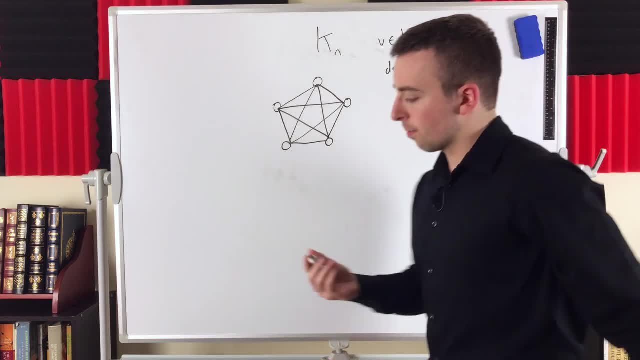 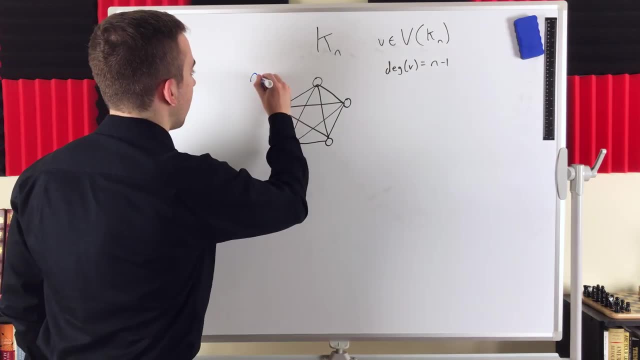 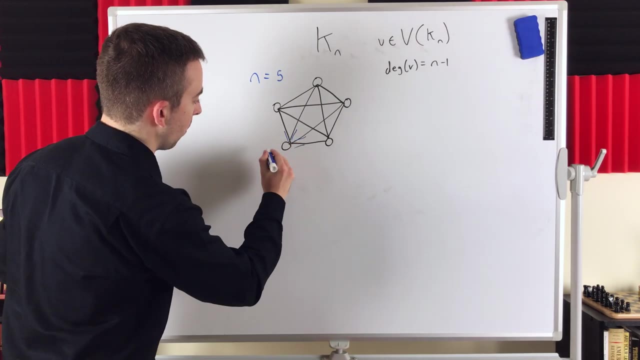 minus one other vertices, And we can see that in this complete graph here. Let me just draw you a few numbers that we can use to change colors. We'll go to blue In this case. n is equal to five. We've got five vertices. The degree of each vertex is four: One, two, three, four. So in this case, 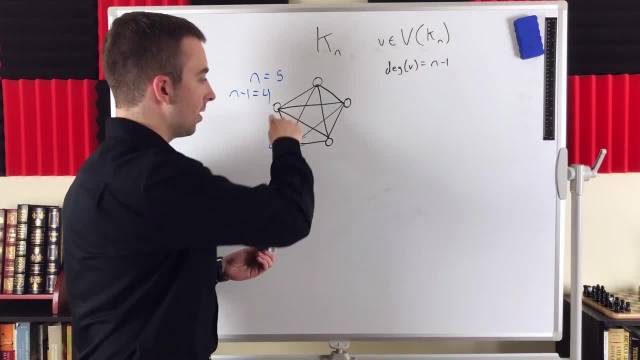 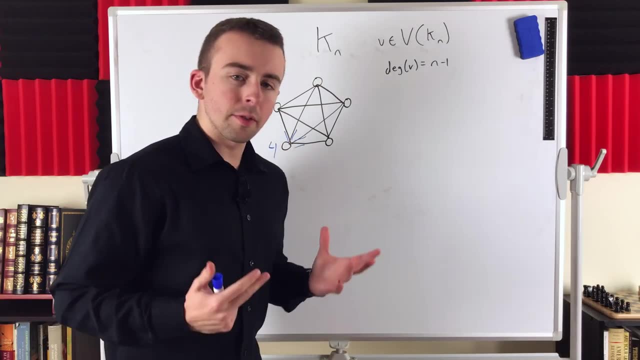 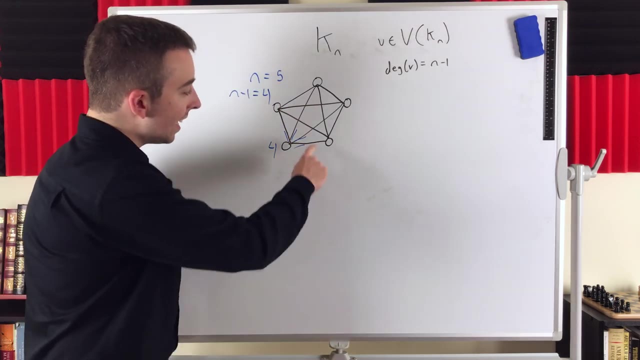 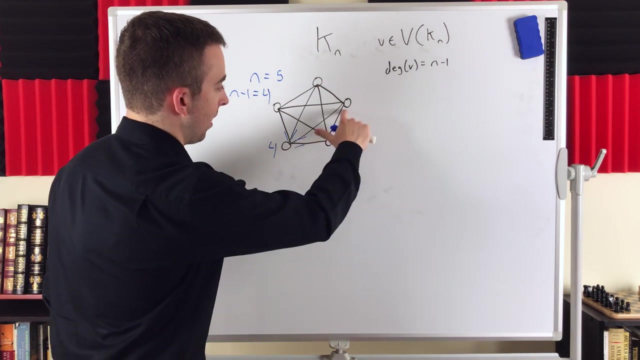 n minus one is equal to four. Each vertex is adjacent to the other four vertices, because that's how a complete graph works. Now, does the degree of a vertex have any relation to edges? Is there any connection we can make? there is. Each edge in a graph is incident to exactly two vertices. right, It's two endpoints. This edge. 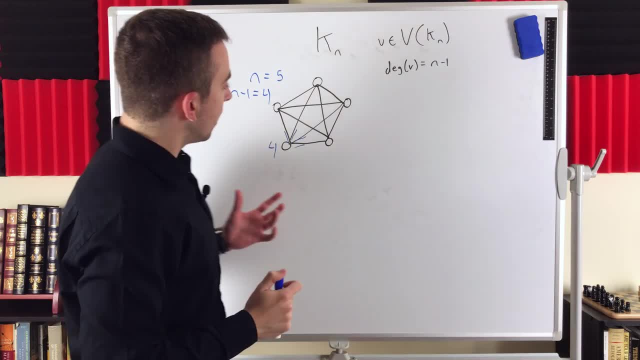 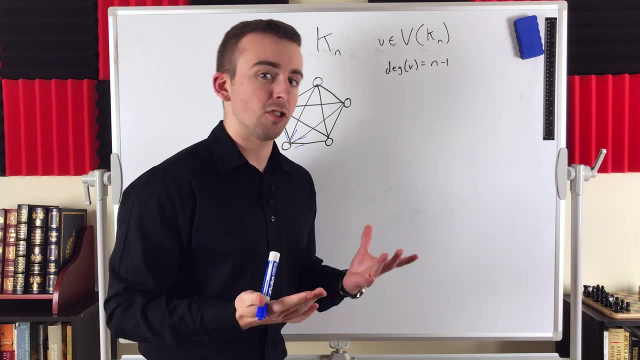 is incident to this vertex and this vertex. So each edge is contributing two to the total degree count of the graph. And that's how we justify the first theorem of graph theory, which you may or may not be familiar with, But if you want to get familiar with that theorem, I'll leave a 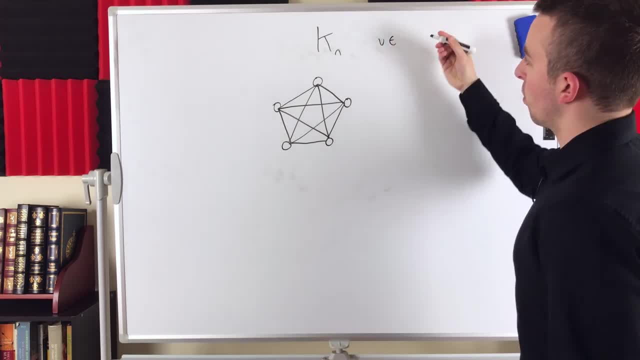 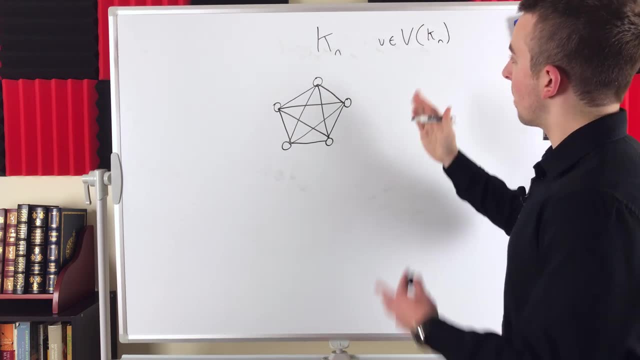 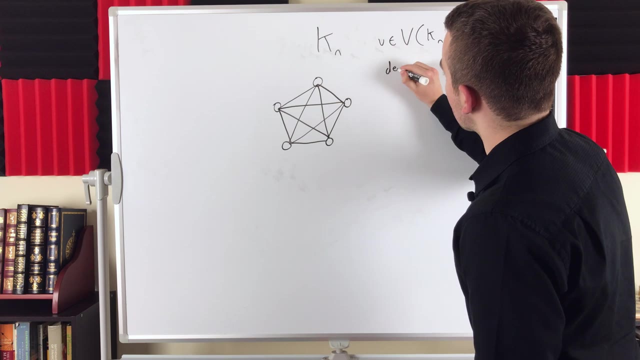 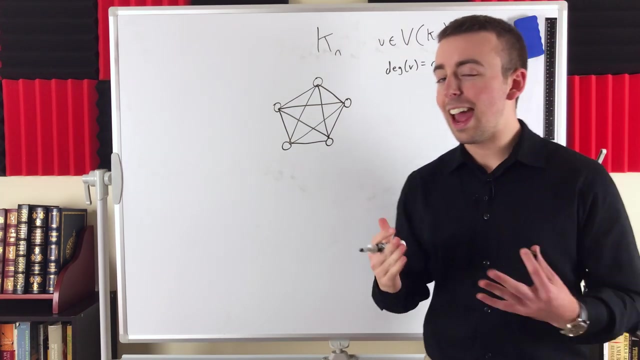 an example of a complete graph. So we'll write that v is an element of the vertex set of k, n. Then v, by definition of complete graph, has to be adjacent to every other vertex in the graph, which means that the degree of v has to be equal to n minus one. It's adjacent to all of the n. 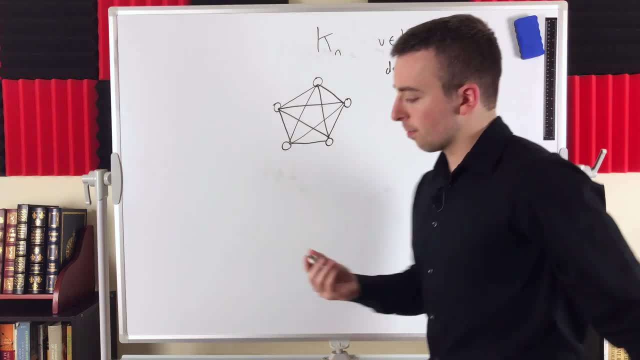 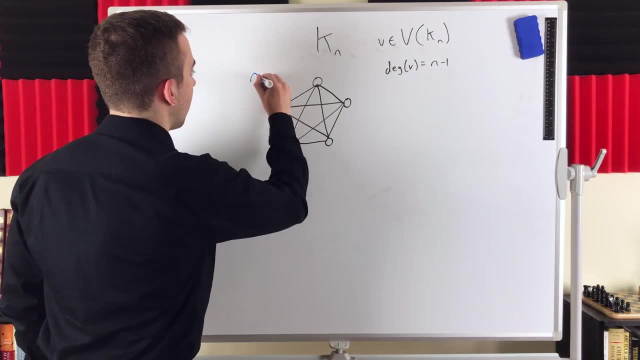 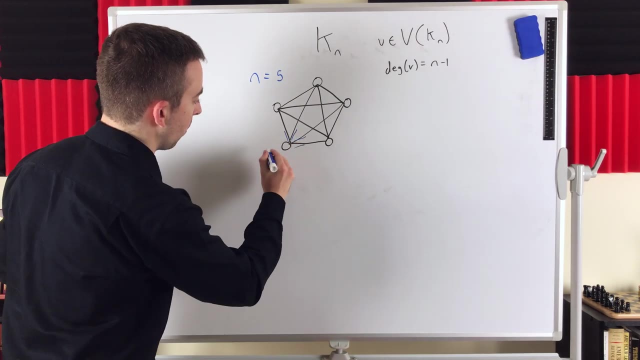 minus one other vertices And we can see that in this complete graph here. Let me just draw you a change colors. We'll go to blue. In this case, n is equal to five. We've got five vertices. The degree of each vertex is four: One, two, three, four. So in this case, n minus one is equal to. 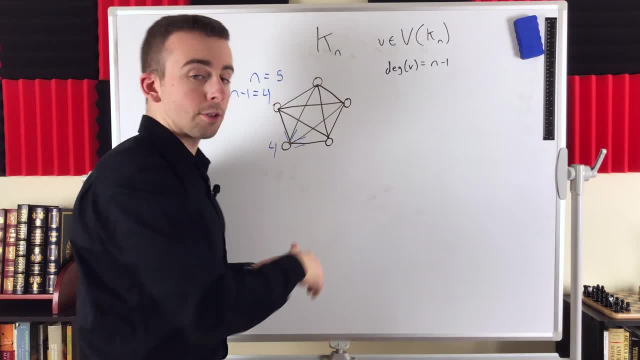 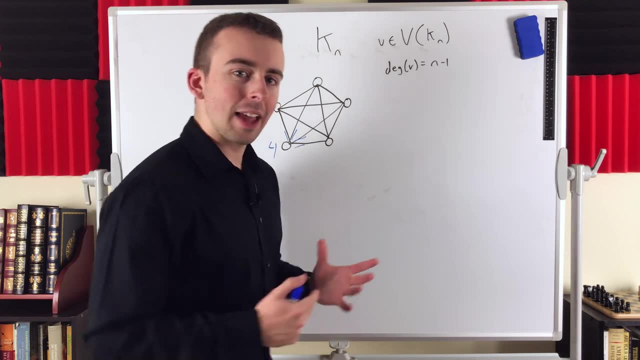 four. Each vertex is adjacent to the other four vertices, because that's how a complete graph works. Now, does the degree of a vertex have any relation to edges? Is there any connection we can make there? Well, there certainly is. We can see that there's a degree of a vertex that has any 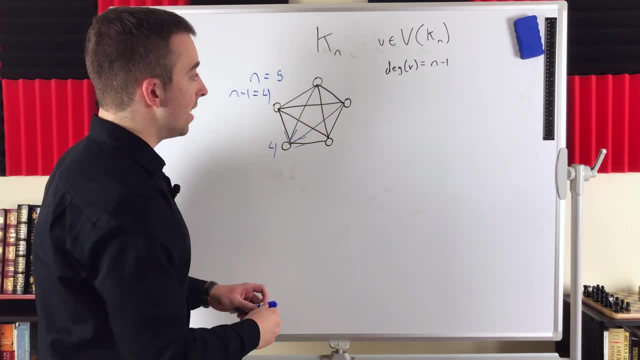 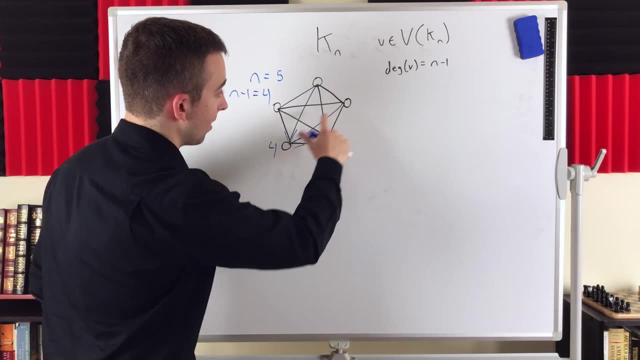 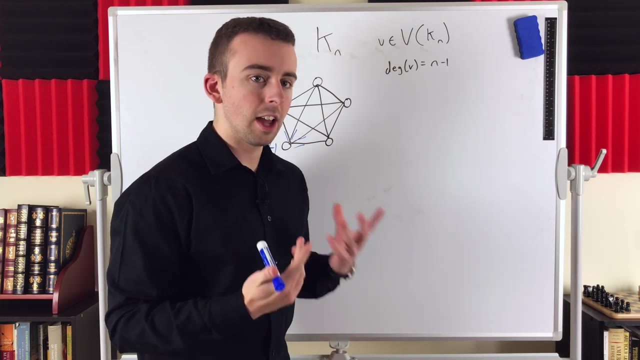 is: Each edge in a graph is incident to exactly two vertices. right, It's two endpoints. This edge is incident to this vertex and this vertex. So each edge is contributing two to the total degree count of the graph. And that's how we justify the first theorem of graph theory which you 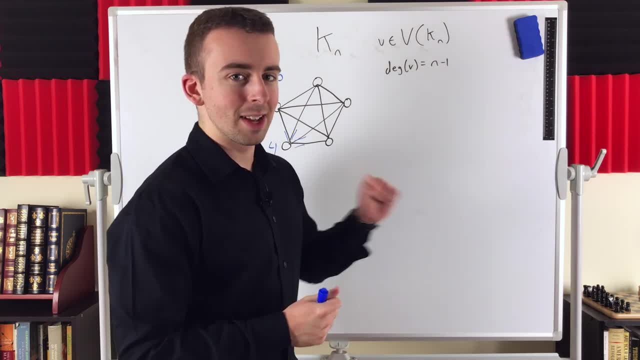 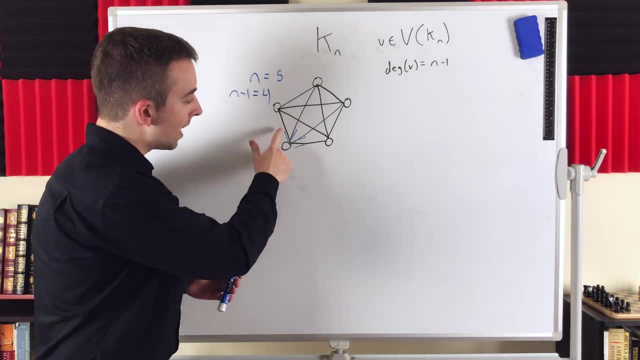 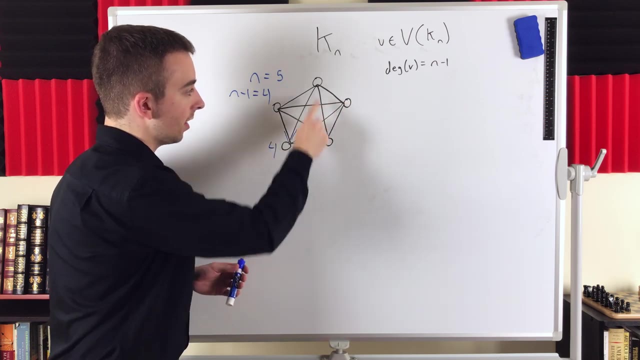 may or may not be familiar with. But if you want to get familiar with that theorem, I'll leave a link down in the description. Now let me quickly recap that point. The degree of a vertex is the number of edges incident to that vertex. Each edge is incident to exactly two vertices, So each edge 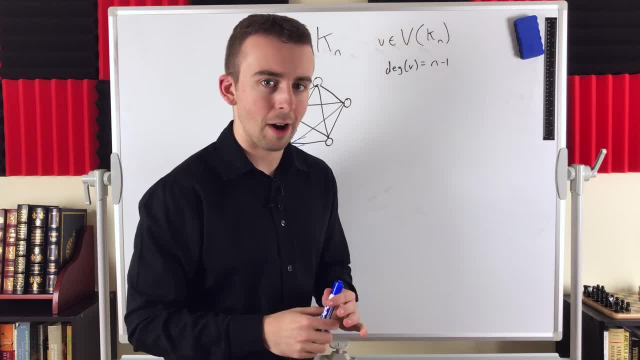 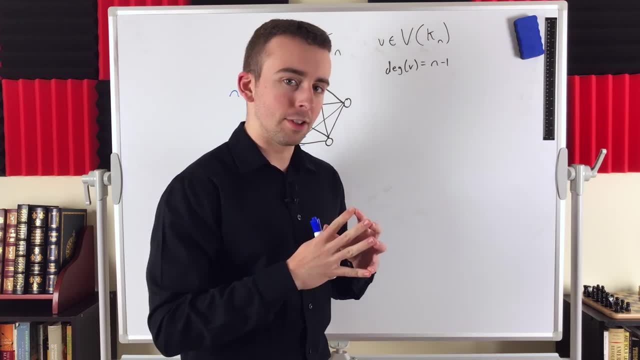 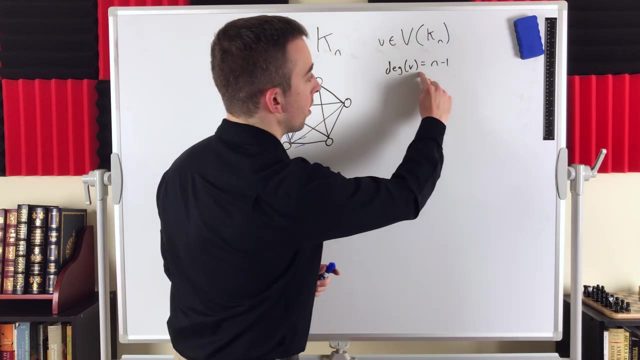 contributes two to the total degree count of a graph. So if we add up all of the degrees- man that train out there is loud- If we add up all of the degrees, we'll get two times the number of edges In the graph. So now we know what the degree of a vertex of a complete graph is, based on the number. 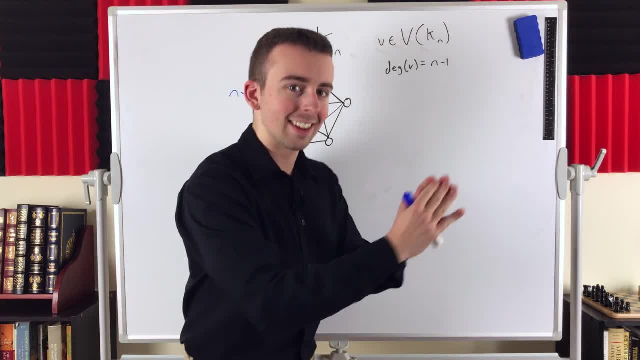 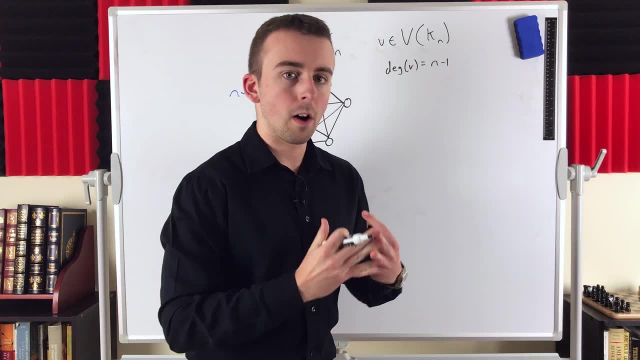 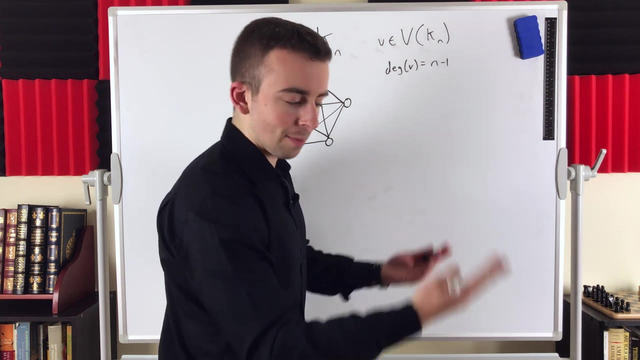 of vertices And we've drawn a connection between that to the number of edges. So let's say we've got a complete graph with n vertices. We want to add up all of the degrees, right? So if we add up all the degrees, that's n minus one plus n minus one plus n minus one, n times because there's n. 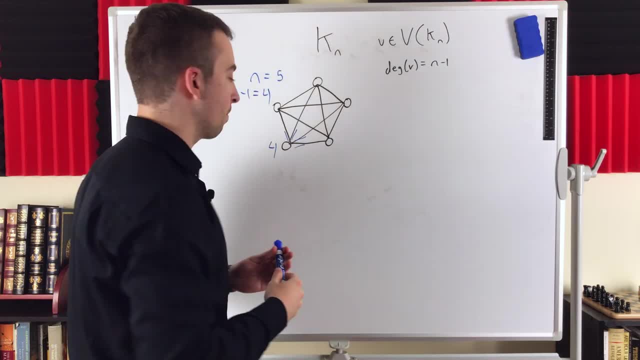 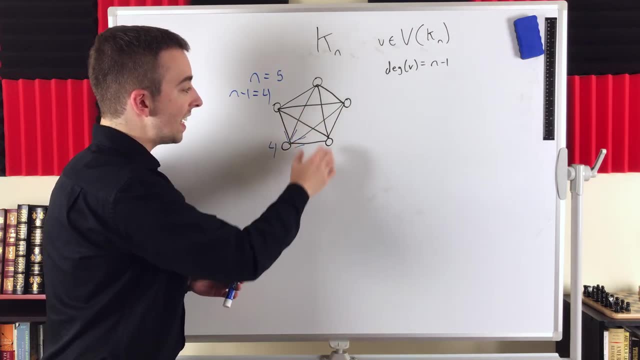 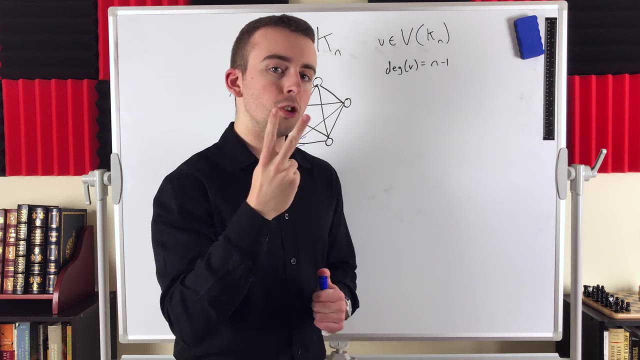 link down in the description. Now let me quickly recap that point. The degree of a vertex is the number of edges incident to that vertex. Each edge is incident to exactly two vertices, So each edge contributes two to the total degree count of a graph. So if we add up all of the degrees, man 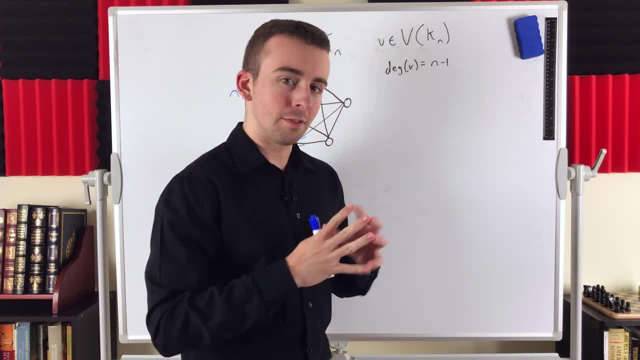 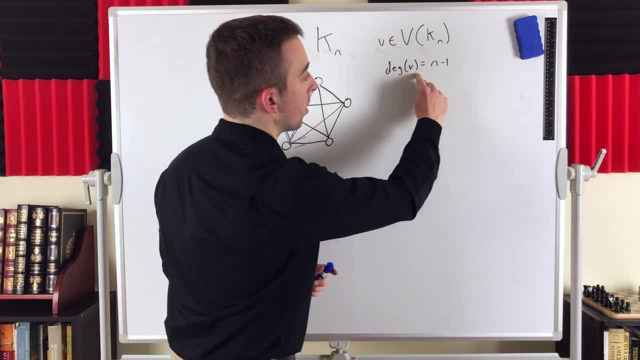 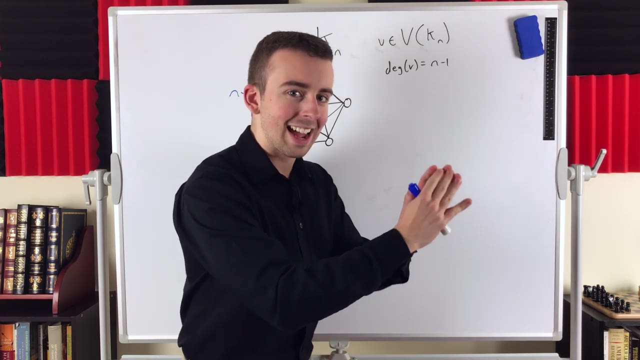 that train out there is loud. If we add up all of the degrees we'll get two times the number of edges In the graph. So now we know what the degree of a vertex of a complete graph is, based on the number of vertices, And we've drawn a connection between that to the number of edges. So let's say we've 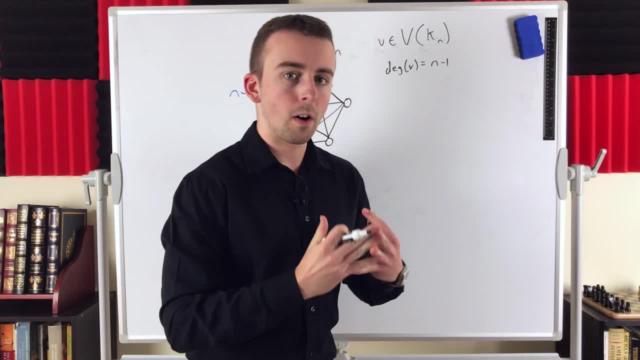 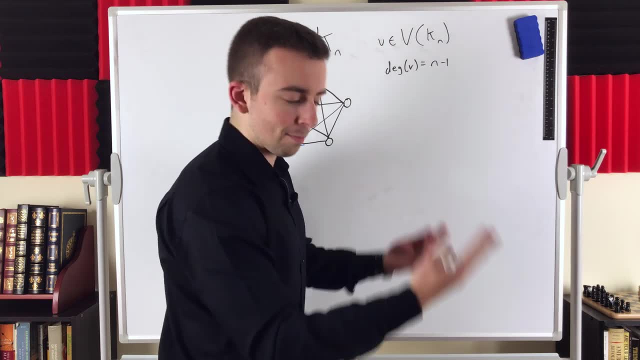 got a complete graph with n vertices. We want to add up all of the degrees, right? So if we add up all the degrees, that's n minus one plus n minus one plus n minus one. n times, because there's n vertices, They all have degree n minus one. So if we add up all the degrees, that's n minus one. 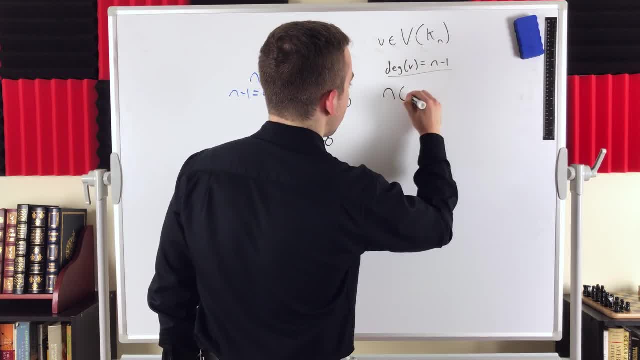 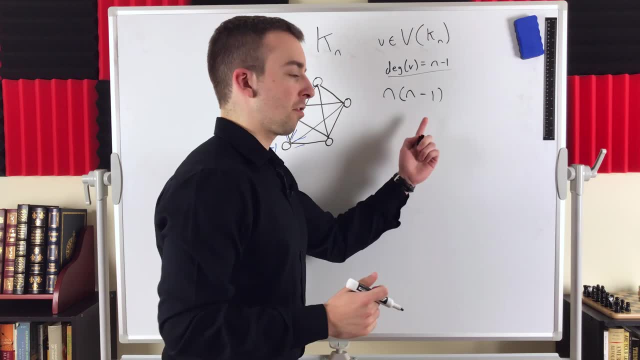 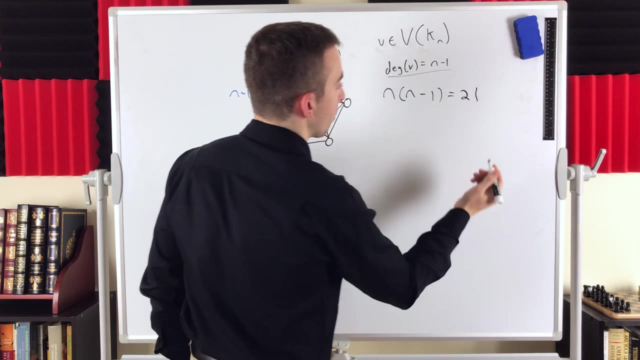 n minus one. So adding up all those degrees would give us n times n minus one, And by the first theorem of graph theory, or by that reasoning I just explained, this is equal to two times the number of edges which we could write like this, two times the cardinality of the edge set. Although 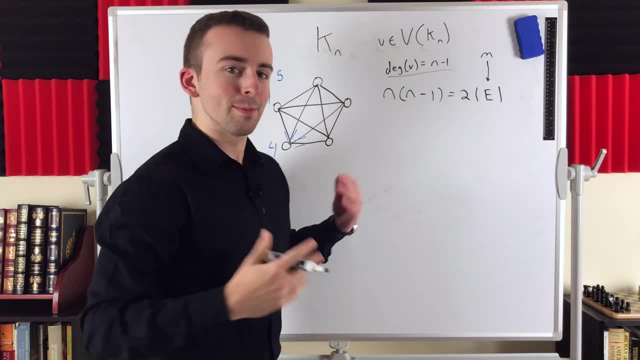 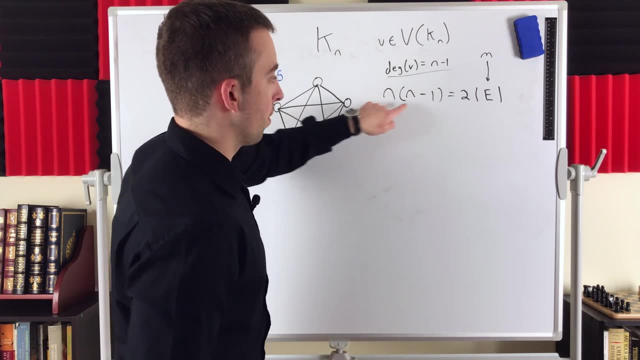 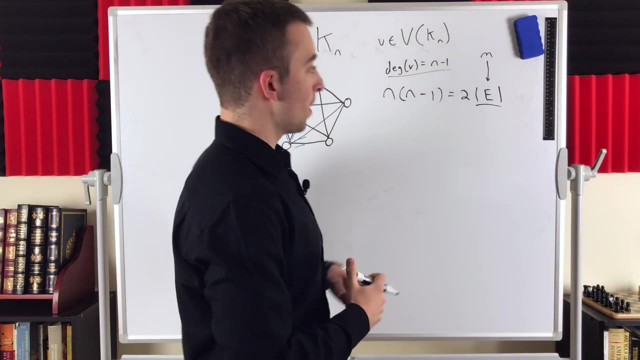 we often just call this m- m for the size of the graph. That's just the letter that we often use. So we add up all the degrees of the vertices in a complete graph. we get two times the number of edges. Now we're interested in the number of edges, right? So just divide both sides by two. 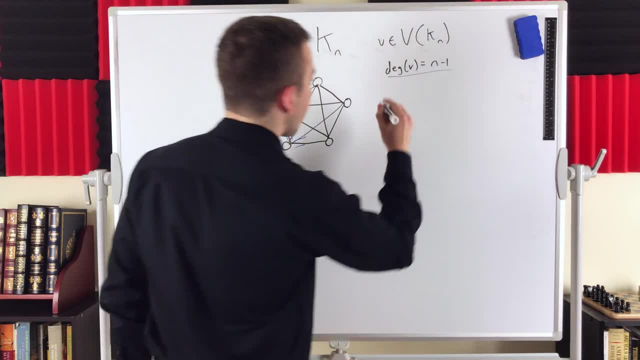 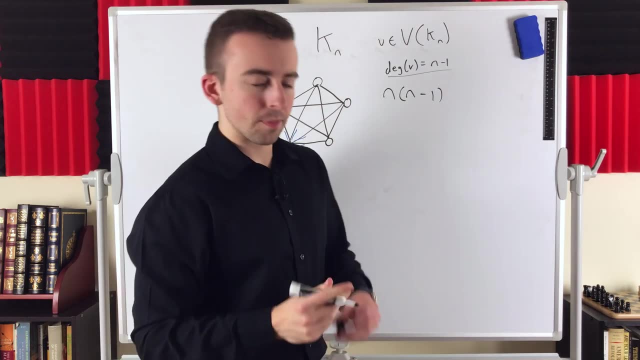 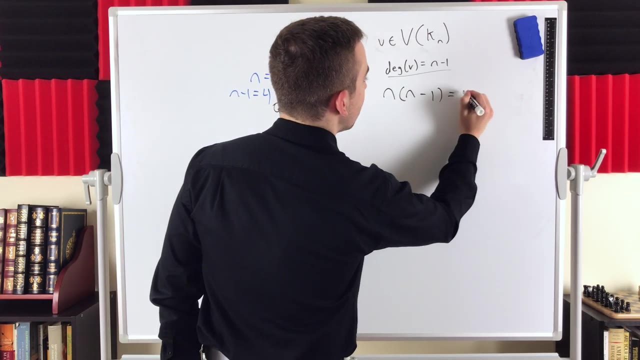 vertices. They all have degree n minus one. So if we add up all the degrees that's n minus one, n minus one. So adding up all those degrees would give us n times n minus one, And by the first theorem of graph theory, or by that reasoning I just explained, this is equal to two times the 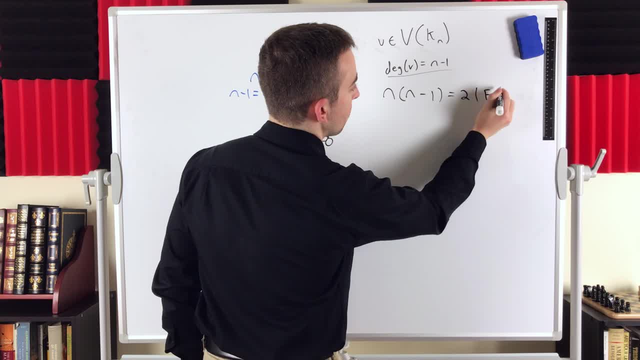 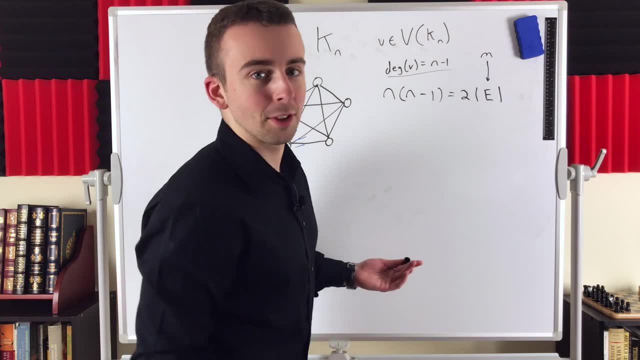 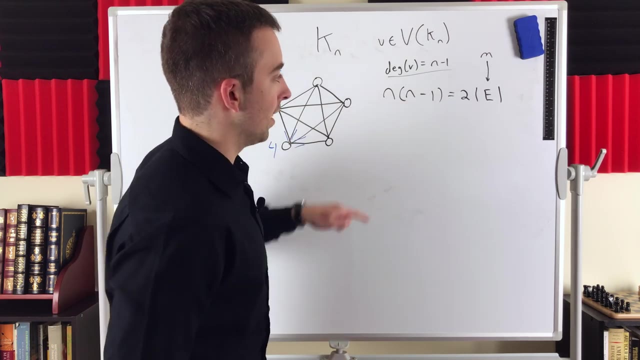 number of edges, which we could write like this: two times the cardinality of the edge set, Although we often just call this m, m for the size of the graph. That's just the letter that we often use. So we add up all the degrees of the vertices in a complete graph, we get two times the number of. 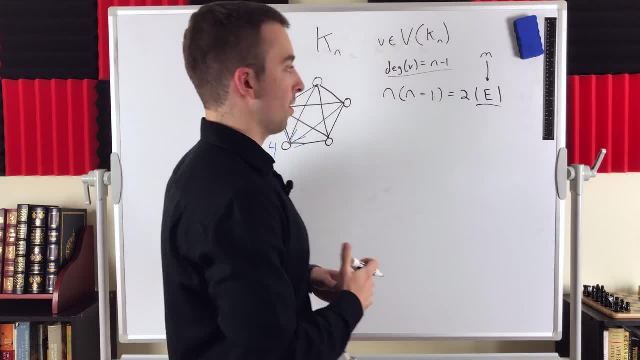 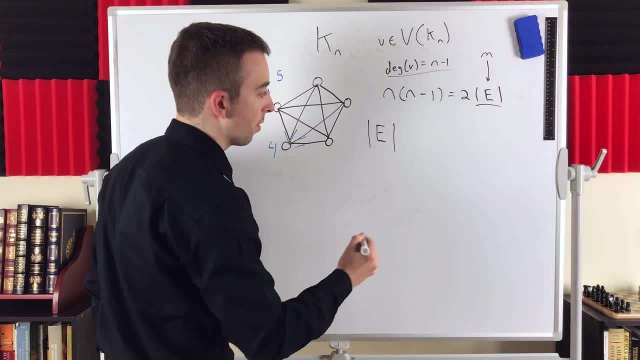 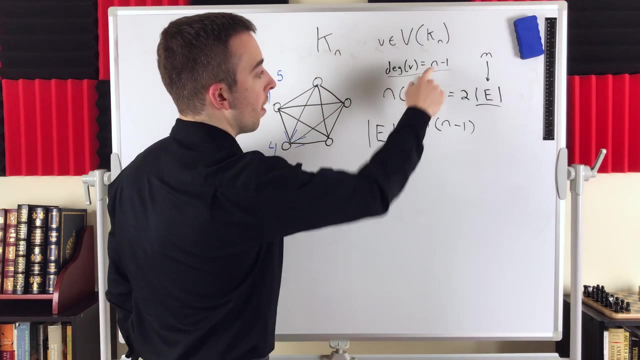 edges. Now we're interested in the number of edges, right? So just divide both sides by two, So we get that the number of edges in a complete graph with n vertices is equal to n times n minus one, which again is the sum of all of the degrees divided by two. When we add it up. 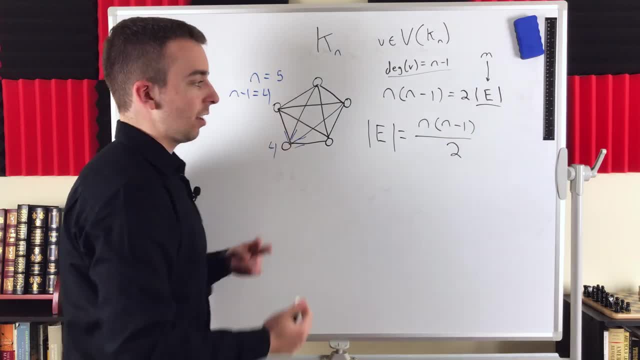 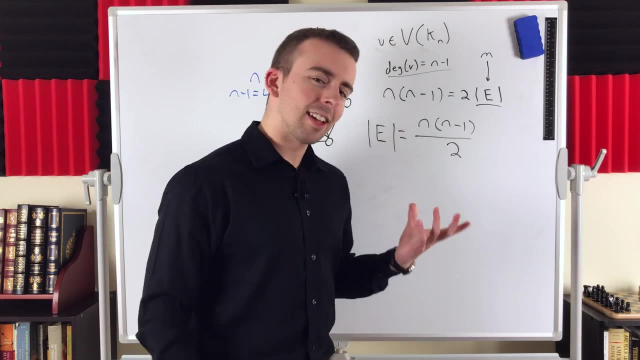 all of the degrees. we are basically counting each edge twice, So when we divide by two, we get the total number of edges. It's pretty beautiful, And if you saw my previous lesson on this topic, then you might notice that this is the same answer, of course, that we got in the 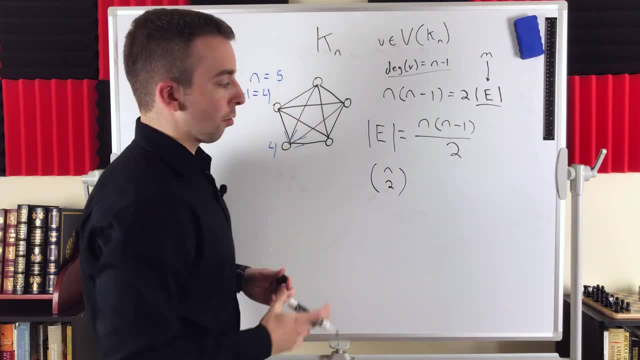 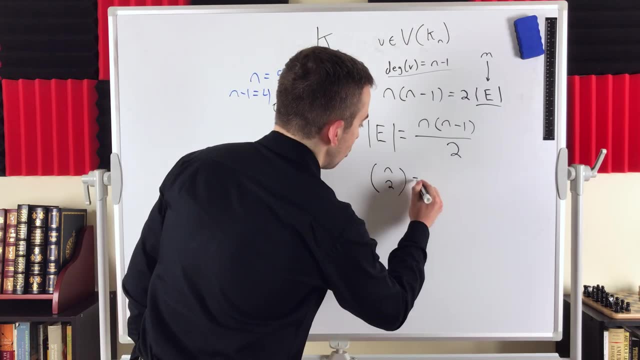 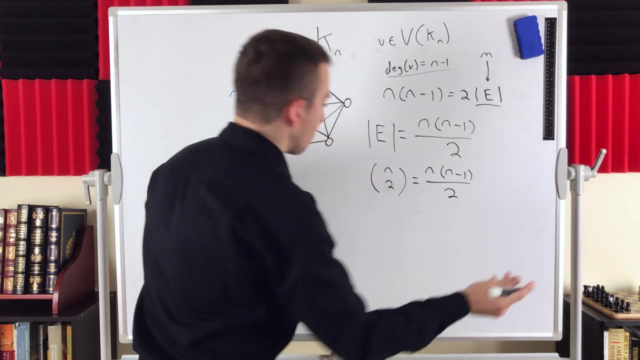 last lesson. In that lesson we used the reasoning that the number of edges in a complete graph on n vertices is a binomial coefficient. n choose two, which, after some simplification, comes out to be the same exact thing. so check out that lesson if you haven't seen it and you're. 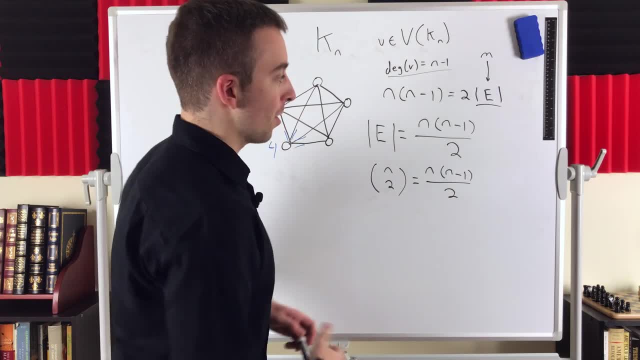 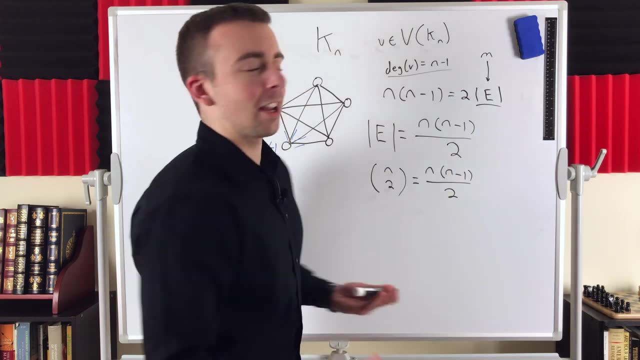 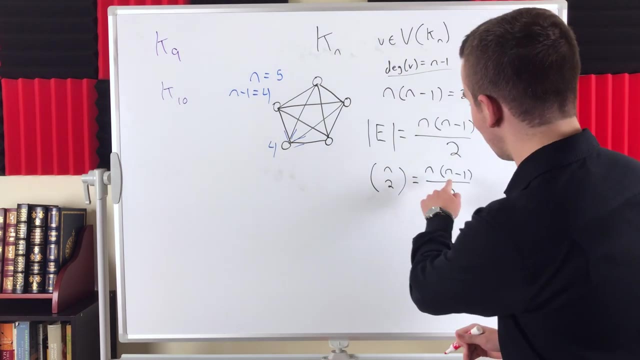 interested, but that is our answer. the number of edges in a complete graph with n vertices is n times n minus 1 divided by 2. pretty cool, hey, sorry, just interrupting because i forgot to include an example in the recording, so let's just quickly apply our result to this example. 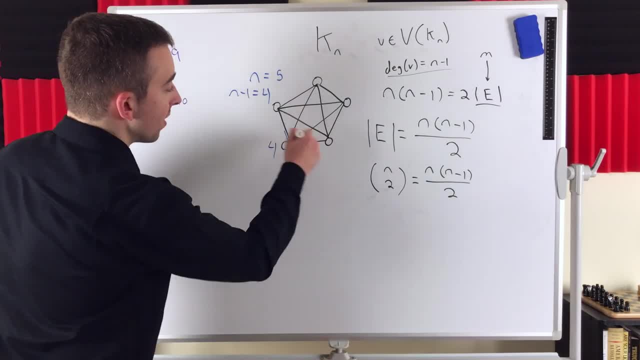 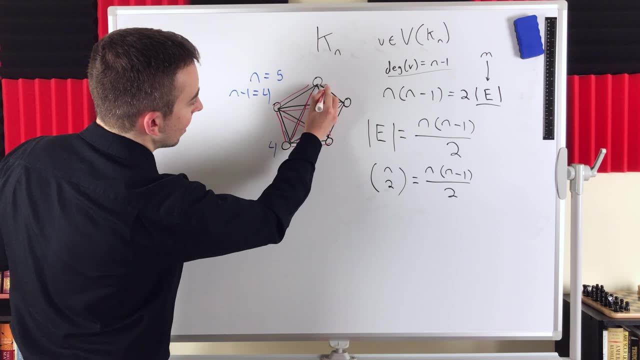 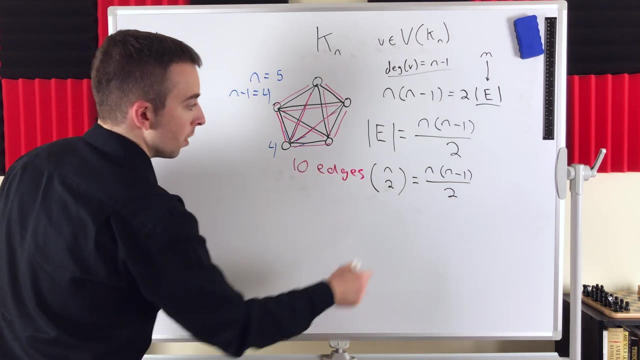 and see if we get the right number of edges. we can see in the example we've drawn out how many edges does this graph have: 1, 2, 9, 10. a little bit messy, but that's how many. it has a total of 10 edges. so, applying this result, we should get the same answer n times n minus 1. 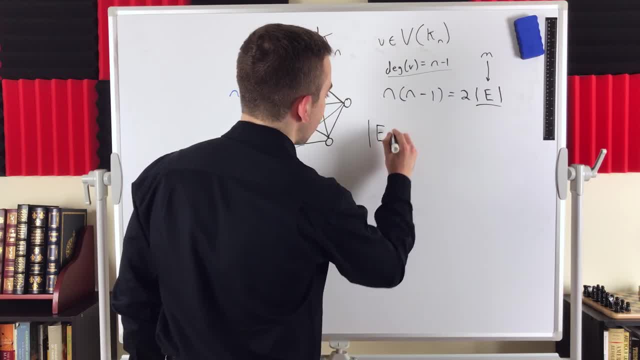 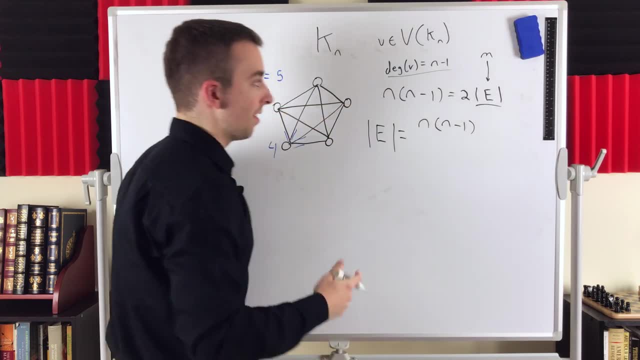 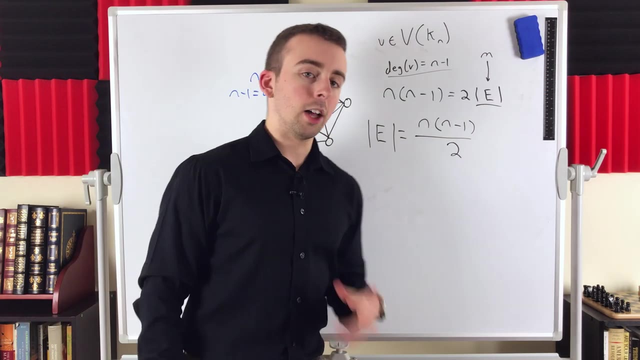 So we get that the number of edges in a complete graph with n vertices is equal to n times n minus one, which again is the sum of all of the degrees divided by two. When we add it up, all of the degrees, we were basically counting each edge twice. So when we divide by two, 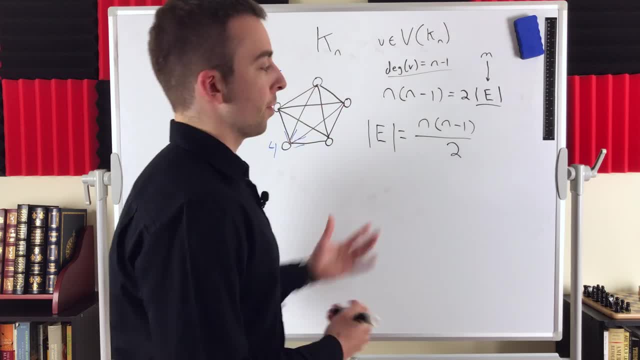 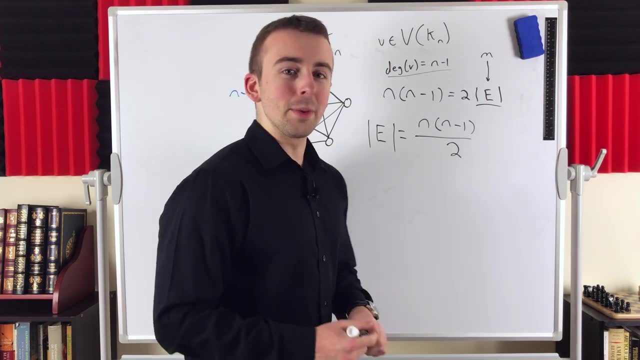 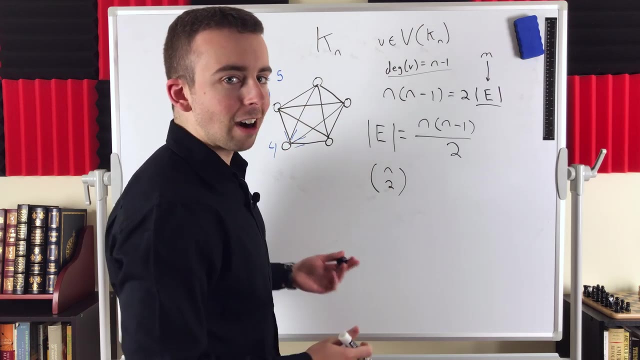 we get the total number of edges. It's pretty beautiful And if you saw my previous lesson on this topic, then you might notice that this is the same answer, of course, that we got in the last lesson. In that lesson we used the reasoning that the number of edges in a complete graph on 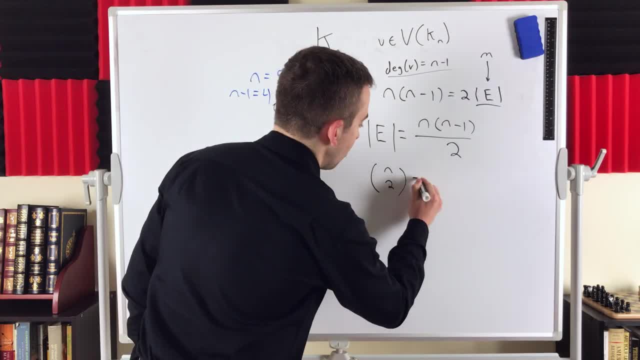 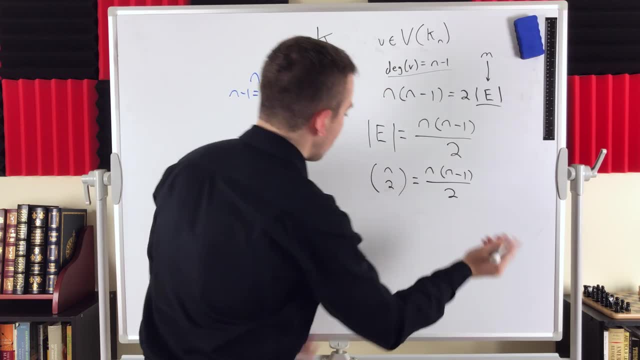 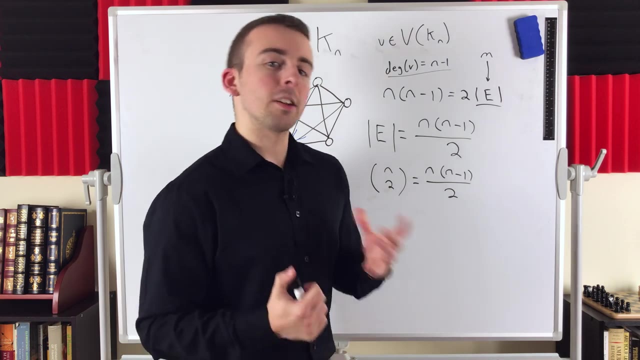 n vertices is a binomial coefficient, n choose two, which, after some simplification, comes out to be the same exact thing. so check out that lesson if you haven't seen it and you're interested. but that is our answer. the number of edges in a complete graph with n vertices: 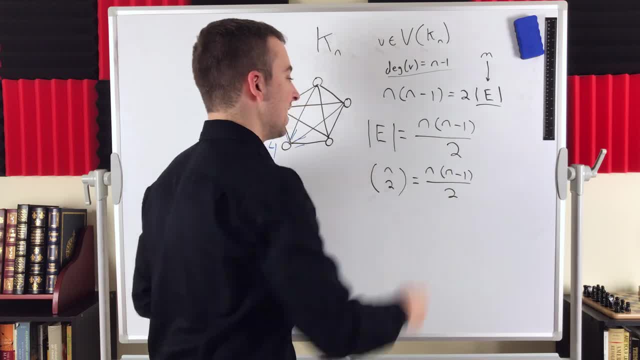 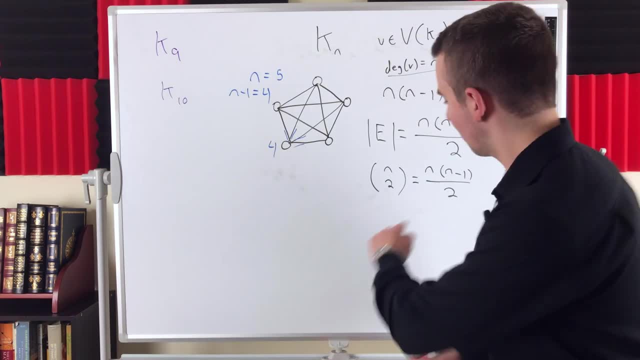 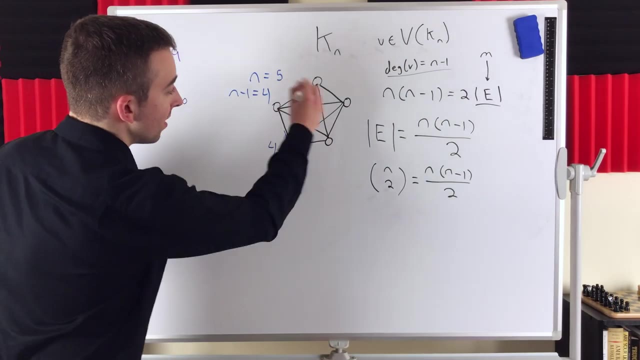 is n times n minus 1 divided by 2. pretty cool, hey, sorry just interrupting because i forgot to include an example in the recording. so let's just quickly apply our result to this example and see if we get the right number of edges. we can see in the example we've drawn out. 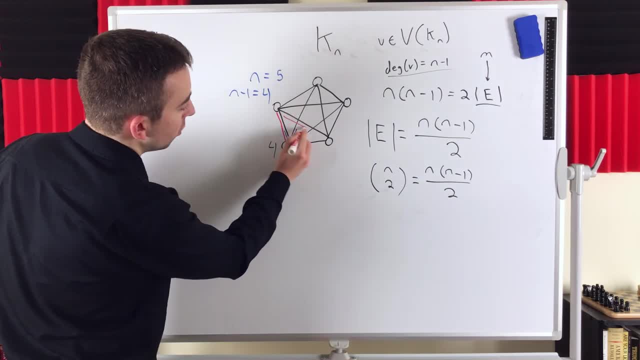 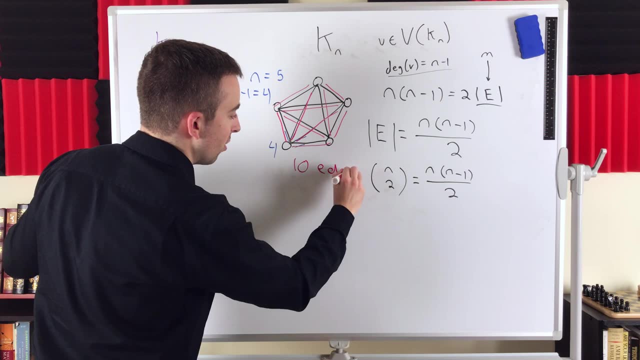 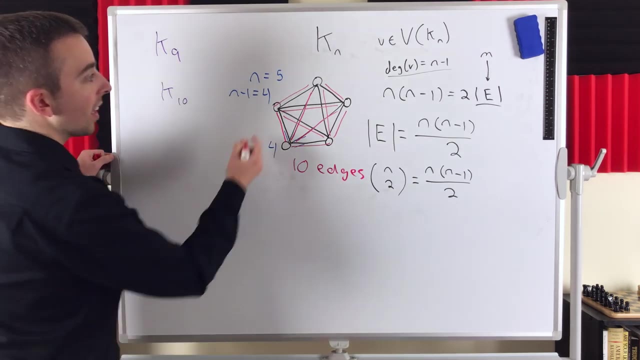 how many edges does this graph have? 1, 2, 9, 10. a little bit messy, but that's how many. it has a total of 10 edges. so, applying this result, we should get the same answer: n times n minus 1. in this case, n is 5, so we'll have 5 times 5 minus 1. 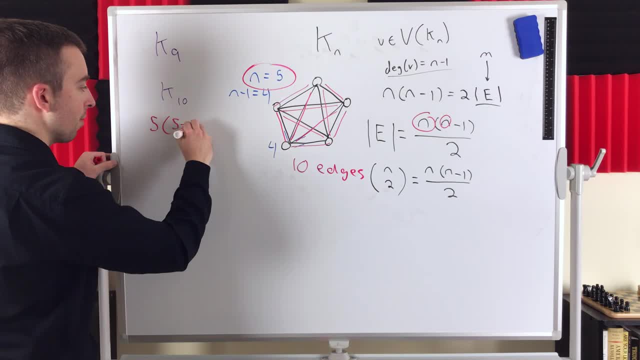 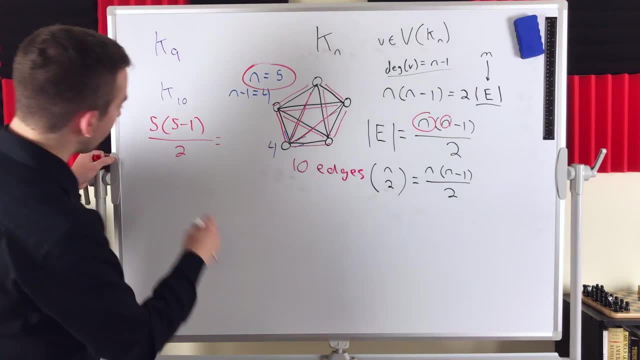 that's, in our numerator, 5 times 5 minus 1, and then, of course, that's divided by 2 and this is the total number of edges, or at least it should be. so we have 5 times 5 minus 1, that's 5 times 4, which is 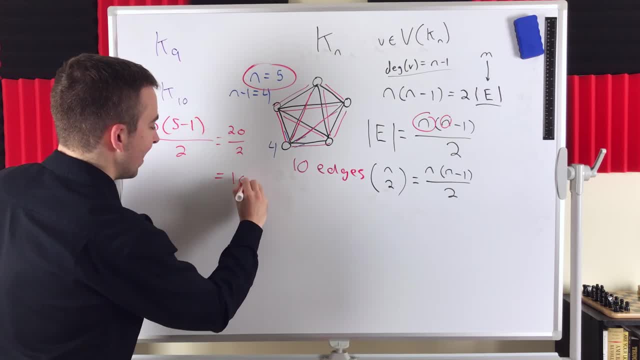 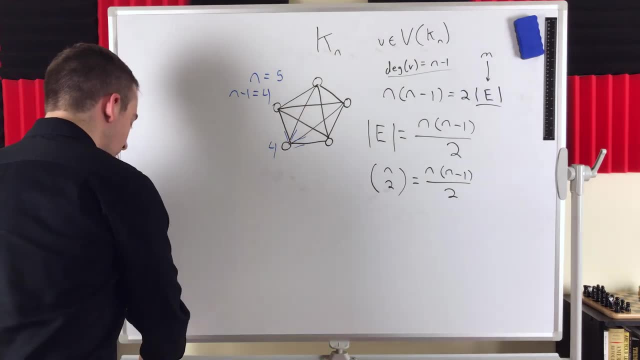 20 divided by 2. hey, look at that, that's 10. it works. just wanted to make sure you had an example. all right, rest of the video now. so let me just leave you with a couple examples to try on your own. find the number of edges in: 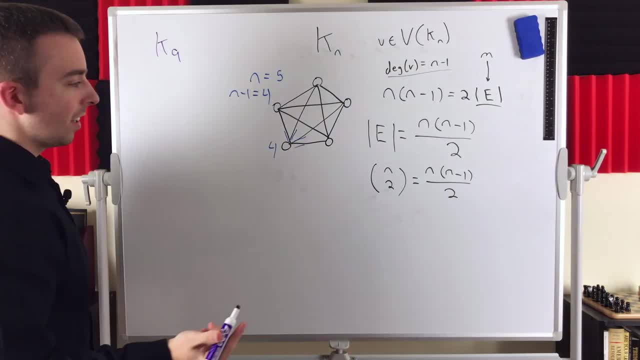 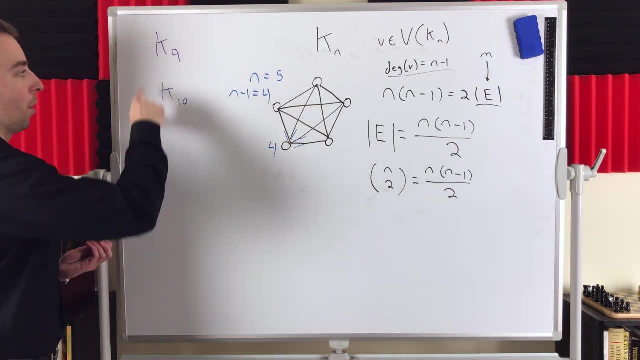 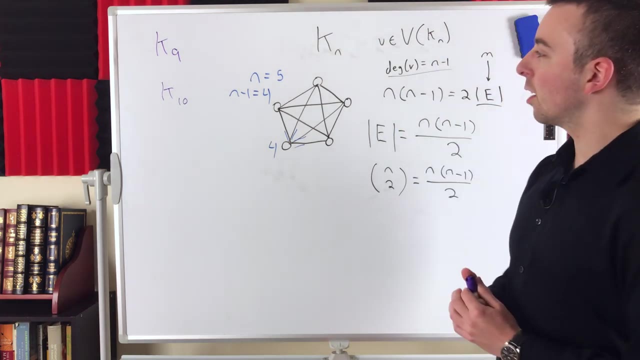 a complete graph with 9 vertices and let's say, in a complete graph with 10 vertices, number of edges in both of these complete graphs. let me know what you get down in the comments and i will of course, leave a solution in the description. so i hope this video helped you understand another way to find.